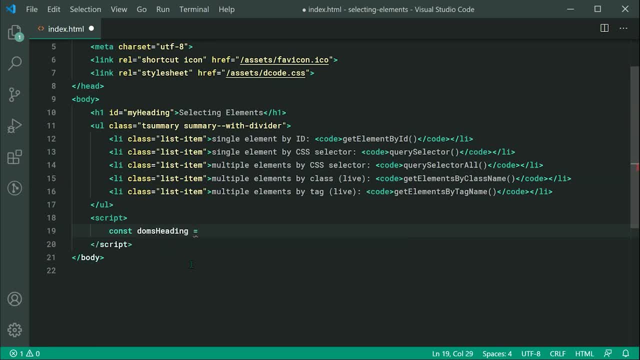 this one Dom's Heading: Hi Dom Digital Dom, Dom, Dom D document. Get ElementById And pass through here MyHeading, just like this. All of this is also case sensitive for those of you who don't know who I don't know, but 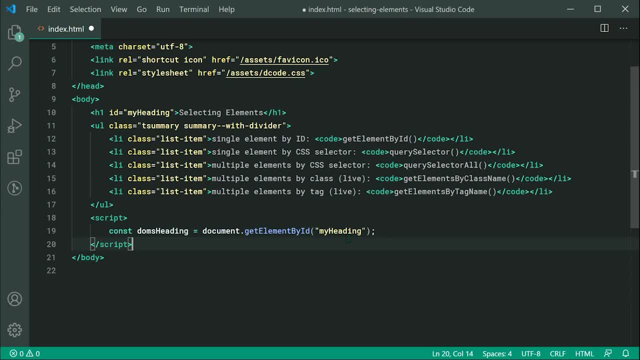 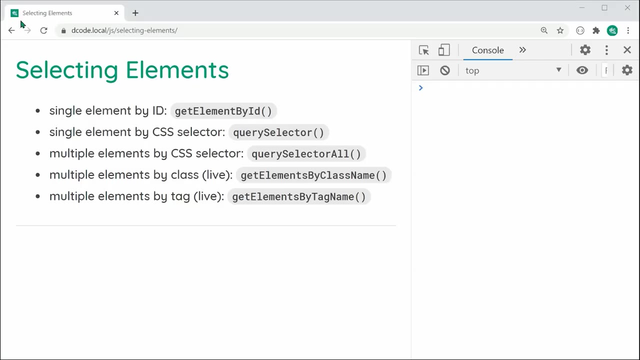 right here. essentially we've selected Dom, the element with the ID of my heading- Quite straight forward. So now, if I was to consolelog doms heading, of course we're going to see in the console doms heading. So I'll just save this right here and refresh and, as we can see inside the JavaScript, 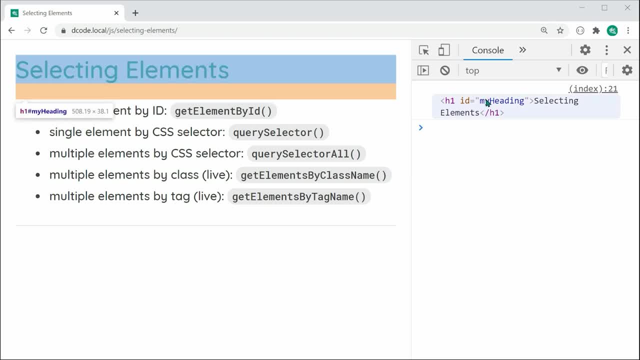 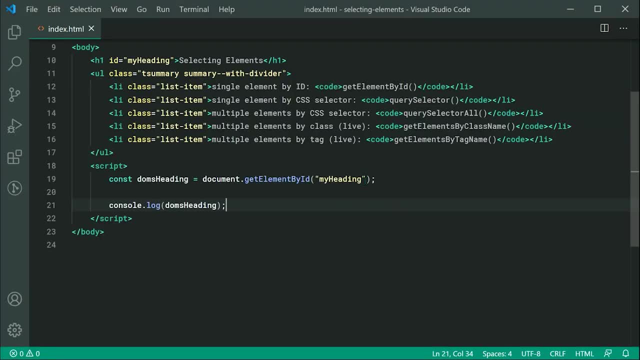 console. we have the h1 tag right there, So that's working perfectly fine. Now what if I was to pass in ID which doesn't exist? For example, if I do my heading 1, that obviously does not exist on the page. Therefore, if I 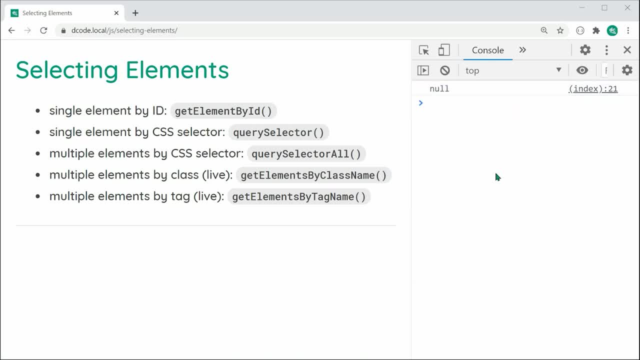 refresh, we get null inside the console, So of course, you're going to have null when your ID doesn't exist. Now, one more important thing in regards to getElementById is that you can only call this method on the document object, So you can only do documentgetElementById. 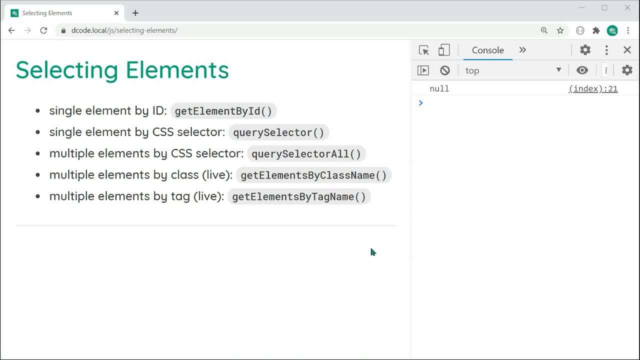 With all of these ones right here, All of these other four ones. these can be ran on actual elements themselves. Okay, so we're going to get to that shortly, but that is all for getElementById. So, moving on to query selector, This one allows you to select an element, So a. 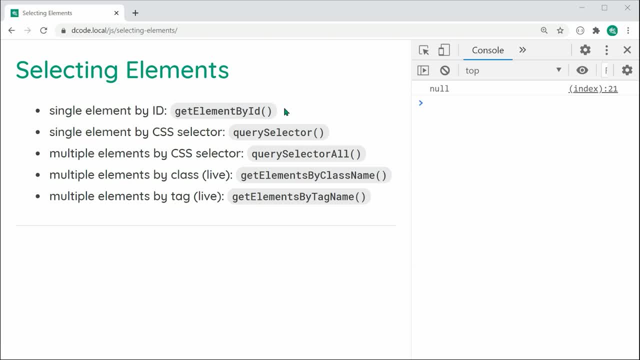 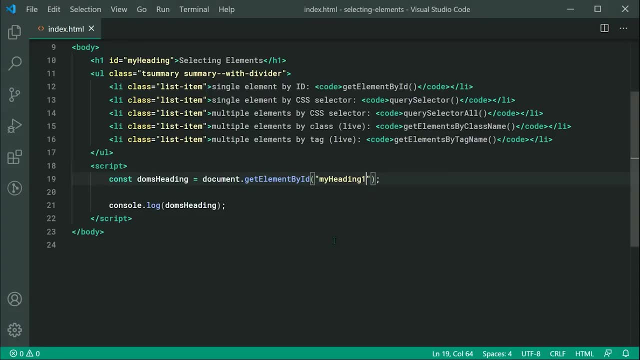 single element, much like the getElementById, but this one allows you to do so using a CSS selector. Okay, so, for example, let's go back inside here now and we're going to be selecting the same thing- the heading- This time. we're going to be selecting the same thing- the heading This time. 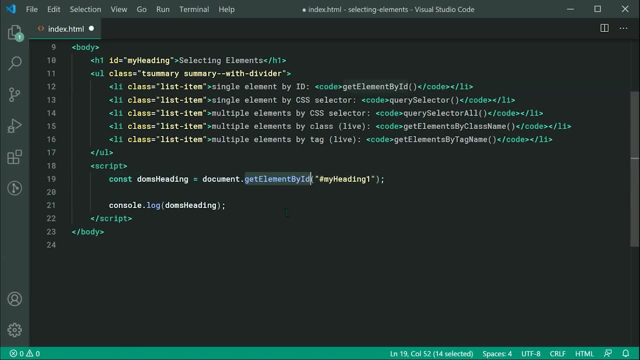 using hash heading and then inside here, query selector, Just like that. So now, right here, we've selected the heading, This time using a CSS selector, with the hash to represent an ID, And that will give us the exact same result, As long as I put. 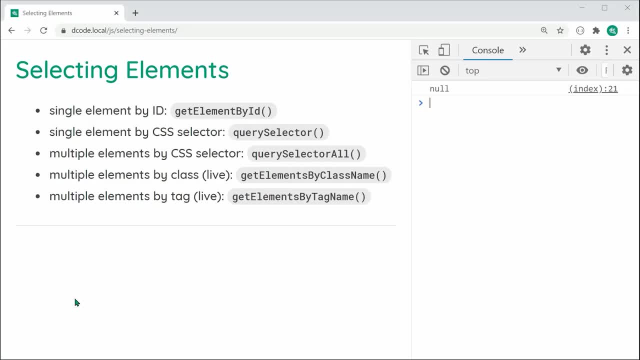 this back to my heading. Let's save this and refresh, and we can see right here we get the same result. We've selected the heading. Now what if I was to once again pass through one, for example? This one is going to give us null. 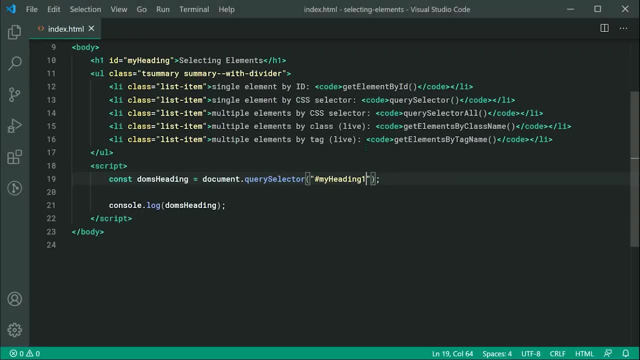 also. Now this becomes interesting because of course, essentially it's going to select the first element which matches the selector. So, for example, if I want to choose the first list item, I can just pass through here a class of list-item, much like I would do within CSS to. 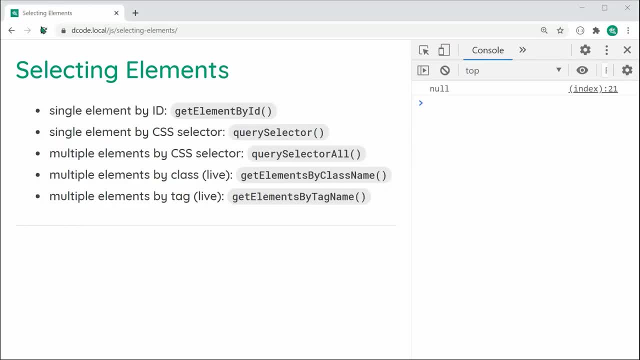 style up this list item, Let's save this and refresh and we can see we get the first list item, Because that, of course. that, of course, is only going to give you one element right here. When it comes to selecting multiple elements through the CSS selector, you can do so using query selector all. 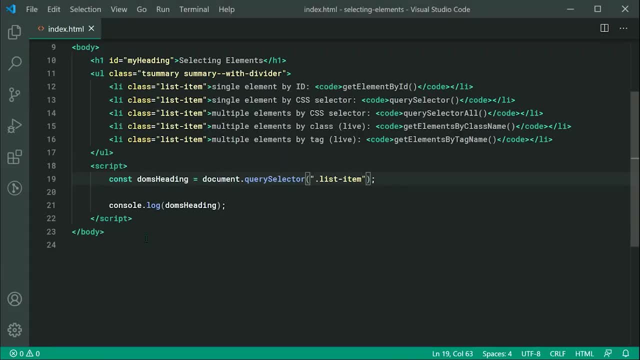 So let's go back inside here. We're going to make a new constant and make this one. Let's just do list items. This will be equal to query selector, then all Okay. so query selector all is going to take in. now our once again list item. So now, if I was to log out. 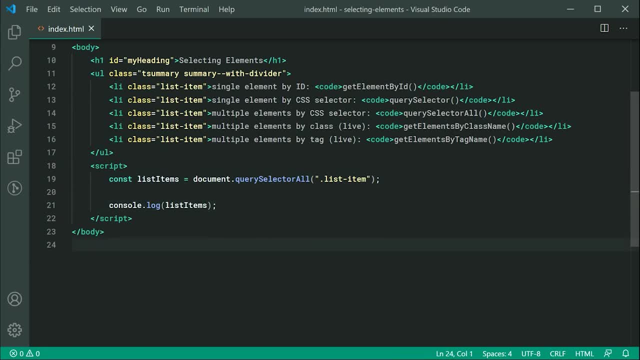 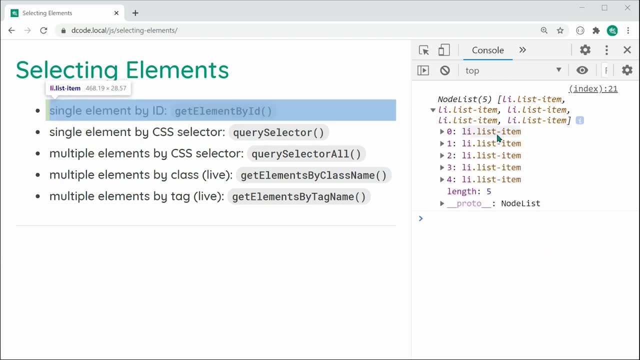 the list items, just like that, and I save this and refresh. we can see right here we get a node list of each one of our list items right here. So each element with a class of list item is present inside here and this node list is an array like object. So 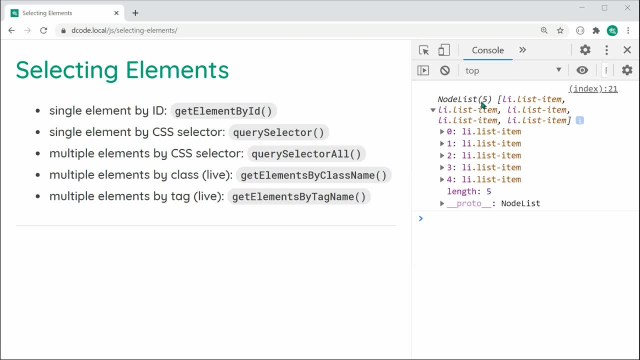 you can access your list items using array syntax. For example, I can say: right here list items, then at index three, it's going to give me the fourth one right there. Okay, so that's quite straight forward. Now, what I was mentioning earlier about the fact that you can call these four: 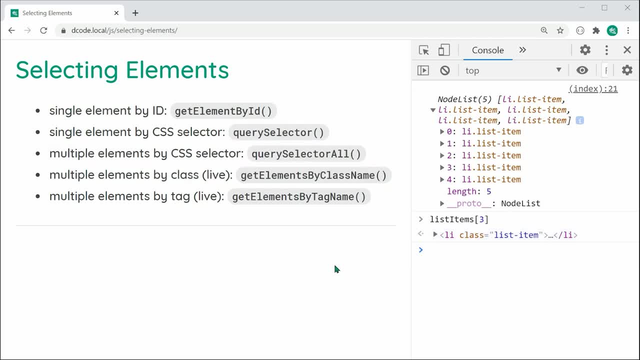 methods on an actual element itself is basically referring to this right here. So if I was to grab the list items at index three, so of course referring to this one right here, I can then say dot query selector on this and I can say: get me the. 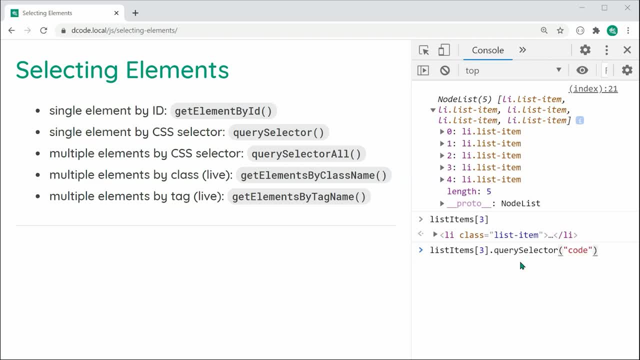 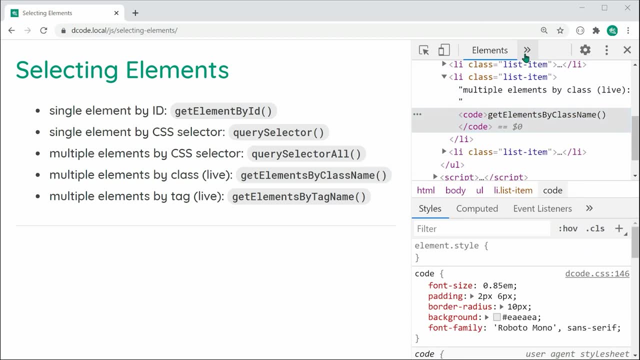 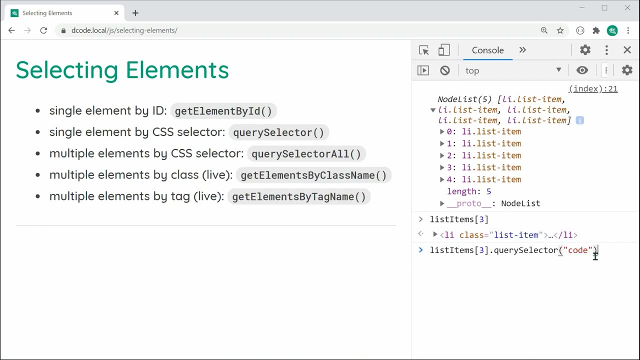 get me the elements for code. Okay, so right here I've got a code tag. Okay, so by calling this query selector on that, it is going to retrieve me the code element or the code tag inside this fourth list item. So now pressing enter, here we can see: 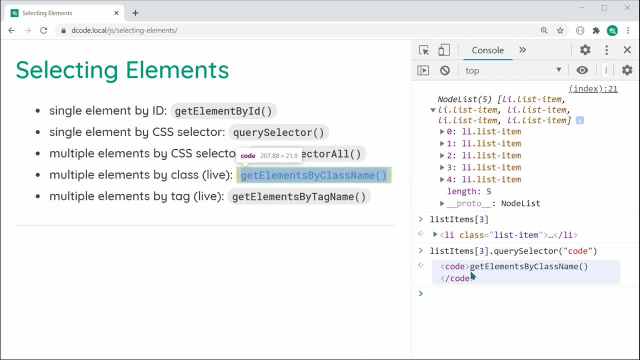 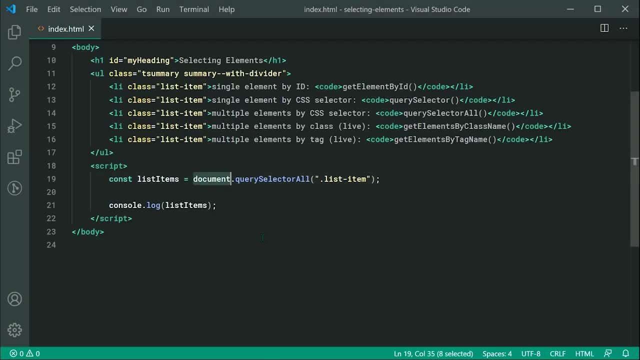 we get that code element right there. Okay, so that's what I mean when I say you can call these four methods on elements themselves, as well as the document right here. So the reason why you may want to call the methods on the actual element itself may be so that you don't actually 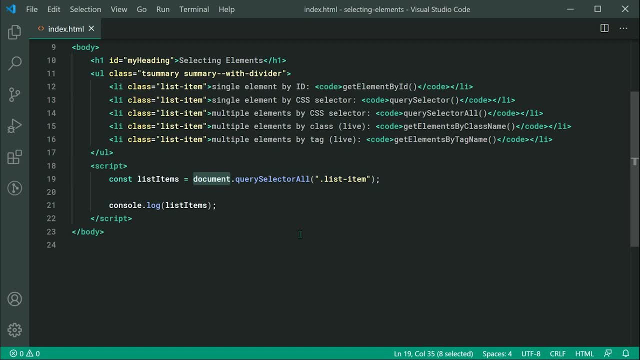 you know you don't select elements that are outside of scope or outside of your particular thing. you know, if you've got some sort of like section or heading or some sort of you know container, you don't want other elements coming into it. you can simply call this: 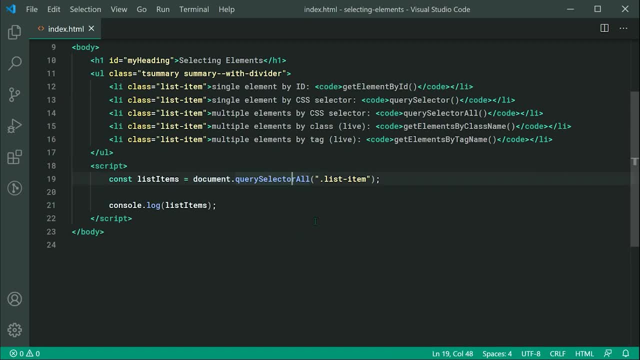 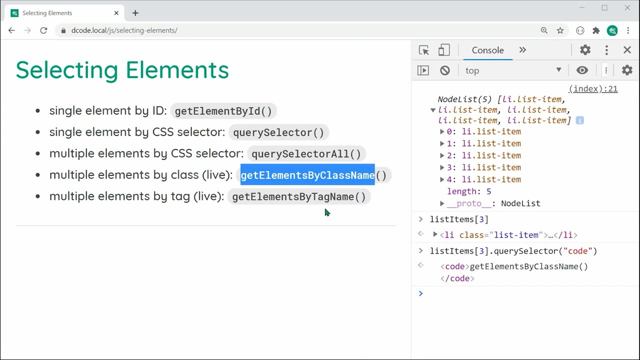 method on the parent, if that makes sense. Okay, so moving on to the last two here. get elements by class name and get elements by tag name. So for these ones right here- you can see in brackets here I've got live. Now, the reason why live is there is because once you 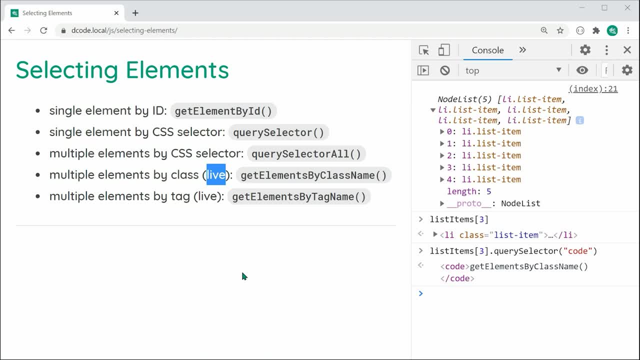 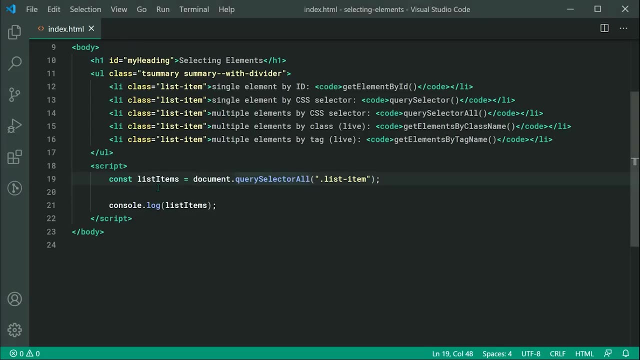 select these elements. so you're going to get an array like structure similar to this right here. Once you select the elements, it is going to give you a live list of those elements. Okay, so right here, for example, we can see I've got the list items constant. so, of course, 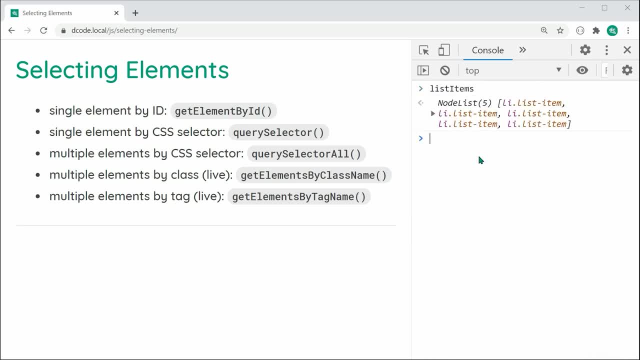 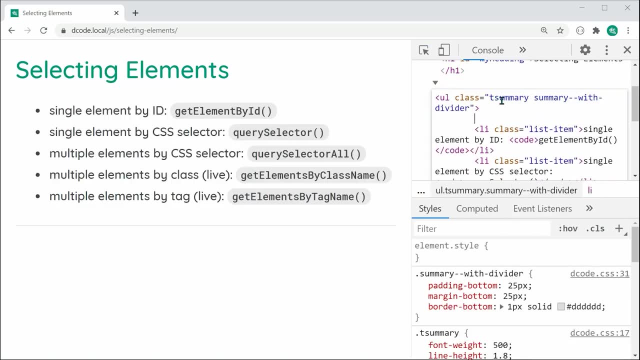 if I was to say list items like this, I'm going to get the node list. Now what if I was to go inside here and I add a new list item inside the inside, the actual inspector here? so I say li, class of list, dash item. then I say decode, for example: 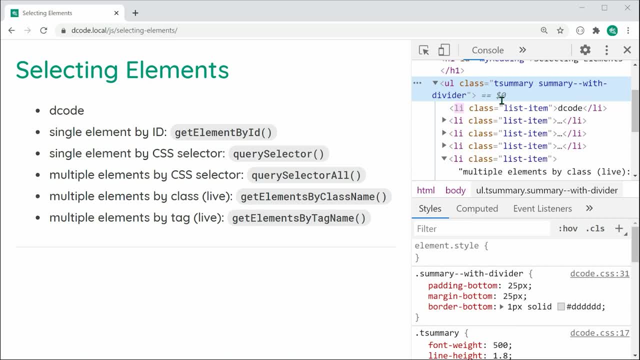 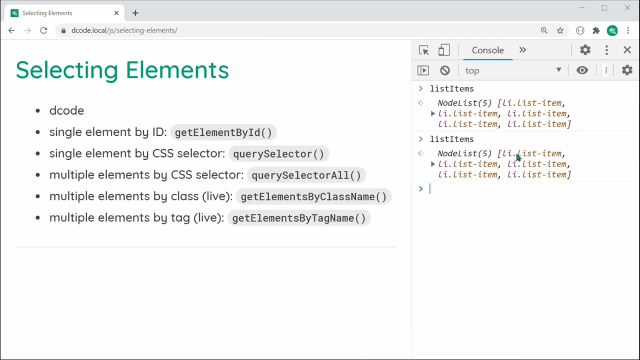 Okay. so if I do this right here, I've now added a new list item. Now, if I go back inside the console here, we can see that list items still contains our five items from four. That is what query selector gives you, Okay. or query selector all gives. 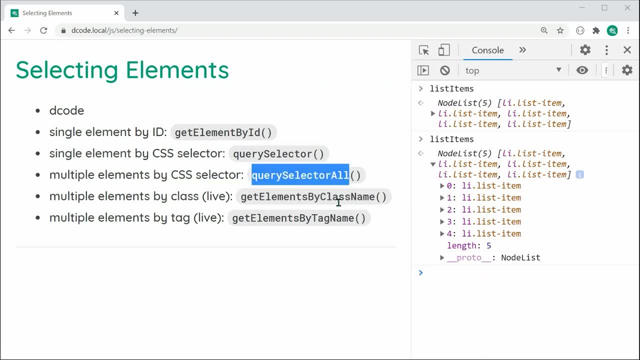 you With the node list here. sorry, with the get elements by class name, this would update as we add a new element, So we're going to be seeing this right now. So let's go inside the text editor and we're going to be using the get elements by class name method. So 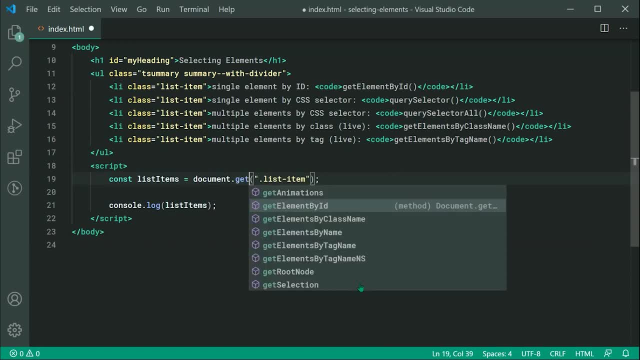 let's go inside here. We're going to say, instead of this, we're going to say: get elements by class name. then we're going to pass through here just the class name. We don't need the dot, because the dot or the period was for the CSS selector. when it comes to 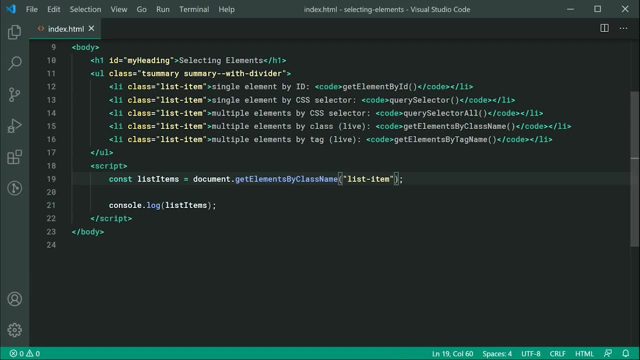 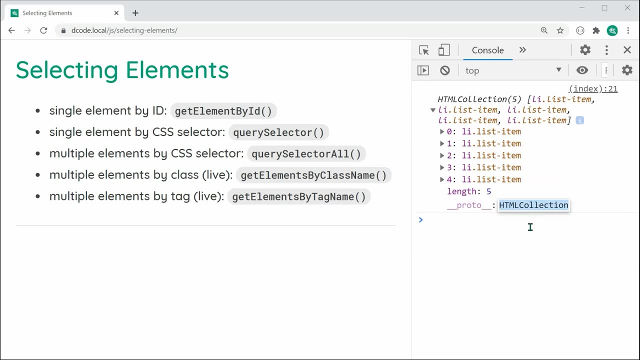 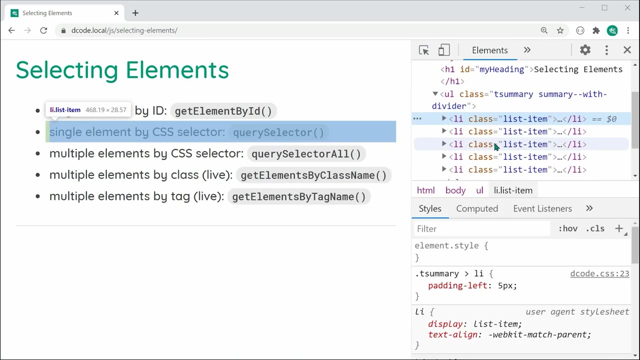 this, you can just pass through the class name. So now, saving this and refreshing, we get right here a similar result. This one is an HTML collection, which means it's going to be live. So let's do the exact same thing where we add the element right here: Edit this and add a new. 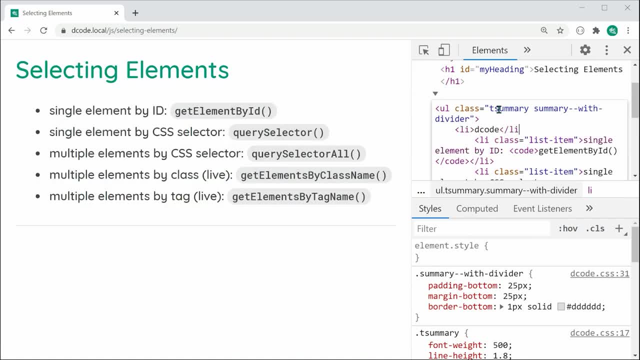 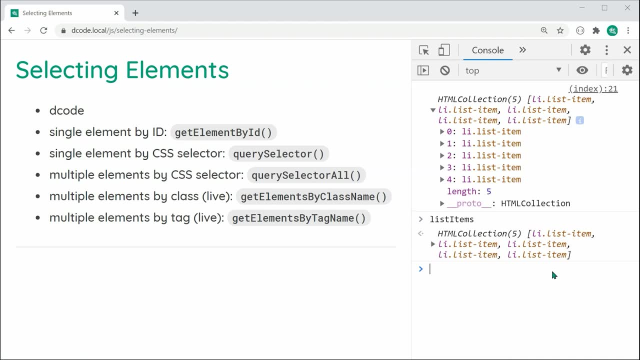 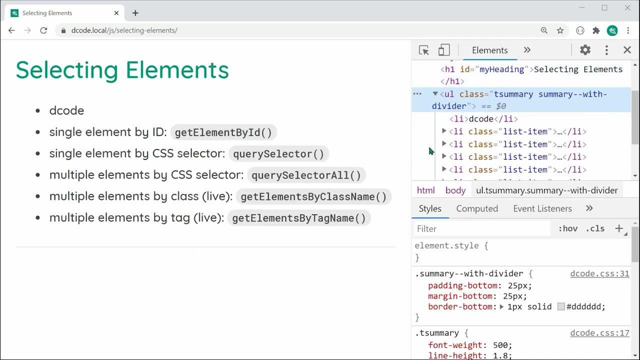 ally tag Pass through decode, press enter. and now, upon going back to the console, if I once again log out our list items, we can see you know what. let's go back and figure out why that didn't work. Let's go inside here. So of course, we need the class. 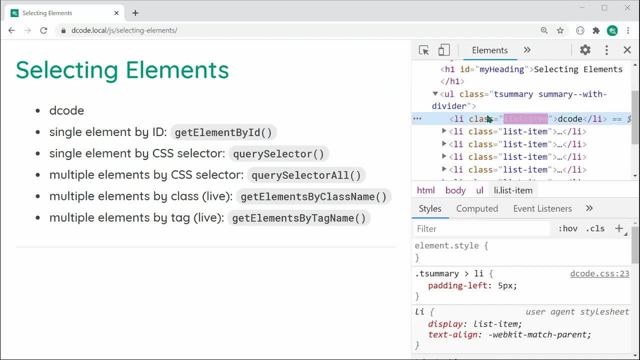 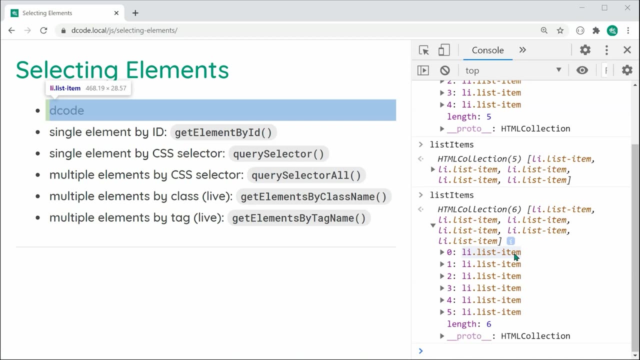 So class list item, Because of course, we're selecting by class name. therefore, we need to pass that class in right there. So let's go back inside here and log out once again. This time we get 6.. So it's included, our top. 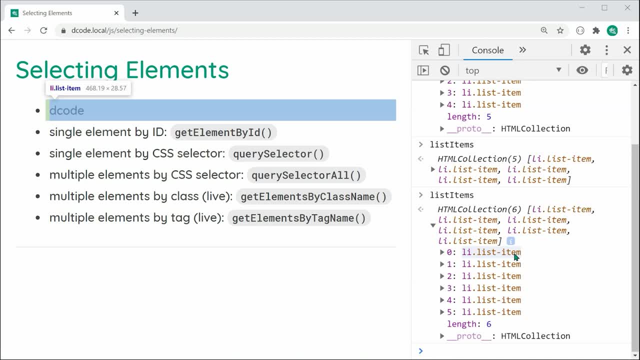 one right there, And that is one of the key differences between selecting your elements through query selector all and get elements by class name. Just keep that in mind. So once you select your elements, you probably don't want to continue selecting them Now. of course, in a similar situation, if I 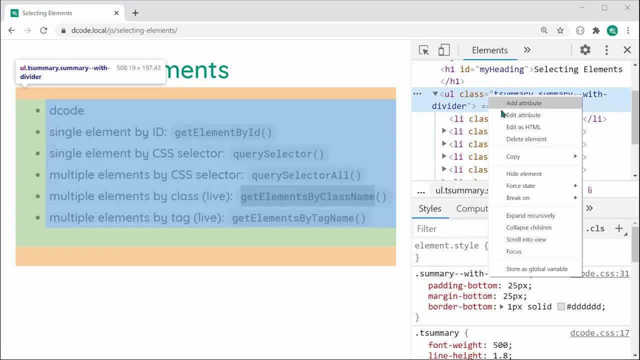 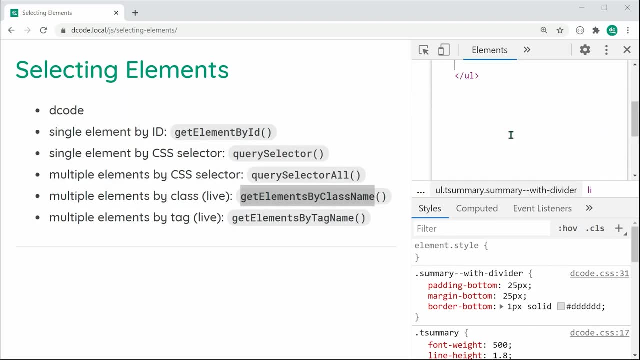 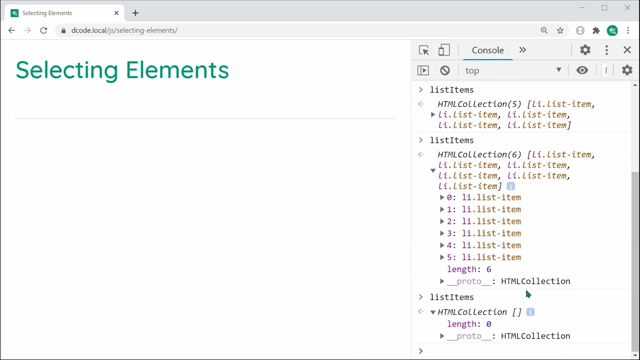 was to go inside here and I actually remove all of my elements from this list right here. So if I say ally and just get rid of all of these list items, Then try it again. we're going to get right here an empty HTML collection. So that is what I mean by it's a live. 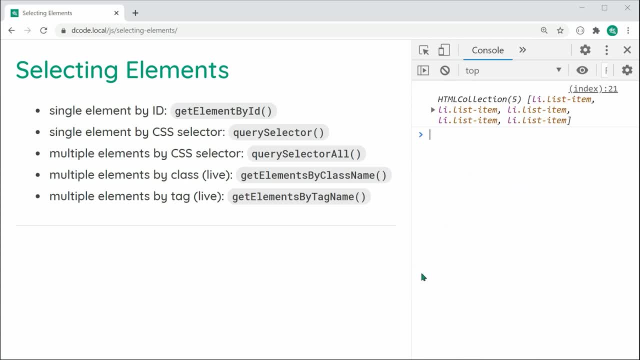 HTML collection. Now, the very last one here- get elements by tag name- is going to, of course, retrieve your elements by the tag name, as the name implies. So this one is going to also give you a live HTML collection, So it's going to work in the exact same way. If I was to go back inside here, 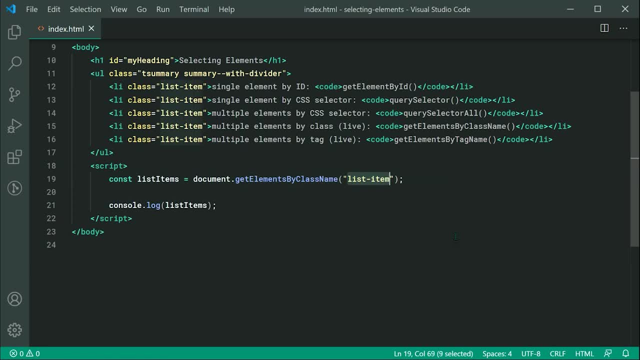 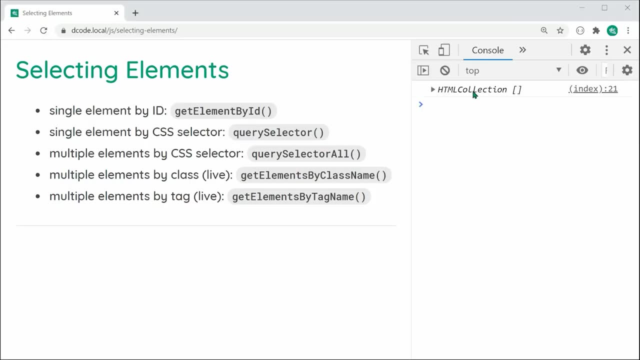 and make this instead of an ally or list item. I'll make this an ally this time, of course, selecting by the tag name, Save this and refresh. We can see right here. we get, of course, an empty collection. Let's figure out why This needs to be. get elements by tag. 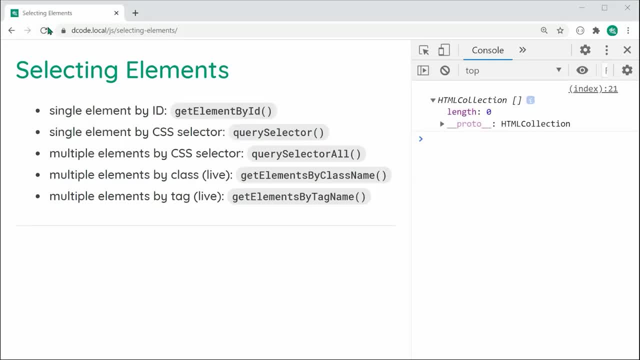 name. Let's try it again and refresh and we see right here we get of course the exact same result and, of course, if I was to add the element right here, it is going to then be live and, of course, appear inside here once I log it out again. Okay so,